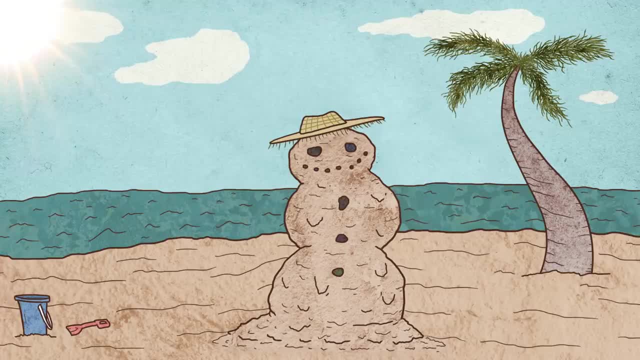 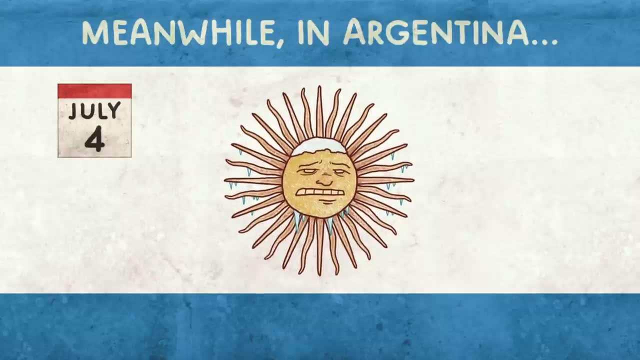 way the world worked, and it was magical. If you had told me back then that one-third of Earth's population had never seen snow, or that July 4th was most definitely not a beach day, I would have thought you were crazy. But in reality, seasonal change, with four distinct seasons, only happens in 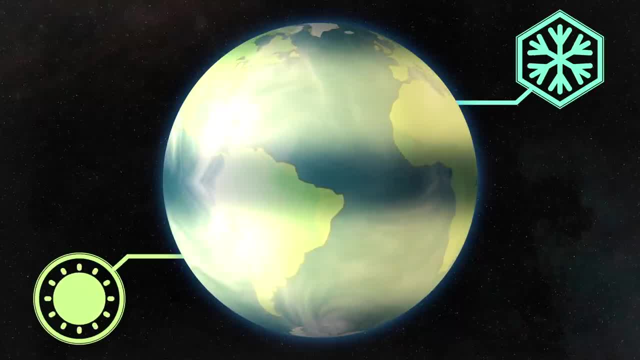 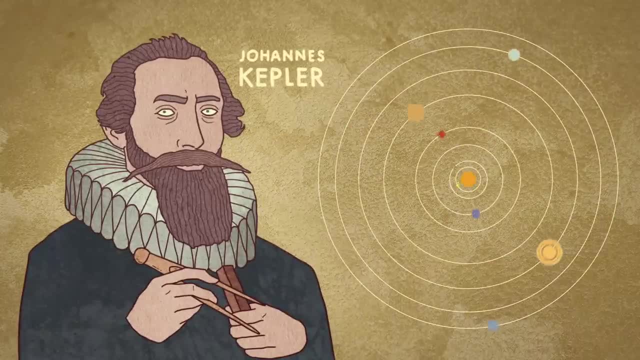 two regions on the planet and even in those two the seasons are reversed, But why? A lot of people have heard of an astronomer called Johannes Kepler and how he proved that the planetary orbits are elliptical and that the sun is not at the center of the orbit. It was a big deal when he 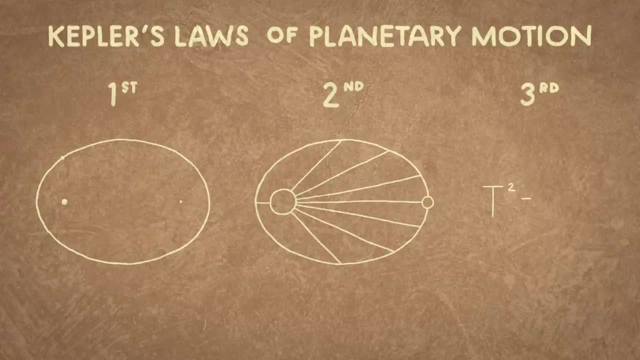 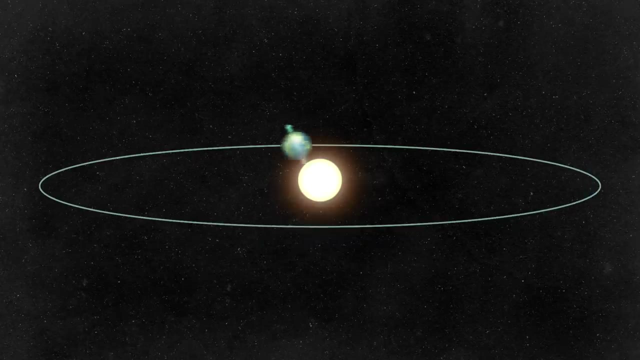 figured this out several hundred years ago. His discovery solved a lot of mathematical problems that astronomers were having with planetary orbit measurements. While it's true that our orbit's not perfectly circular, those pictures in our science books, on TV and in the movies give an exaggerated 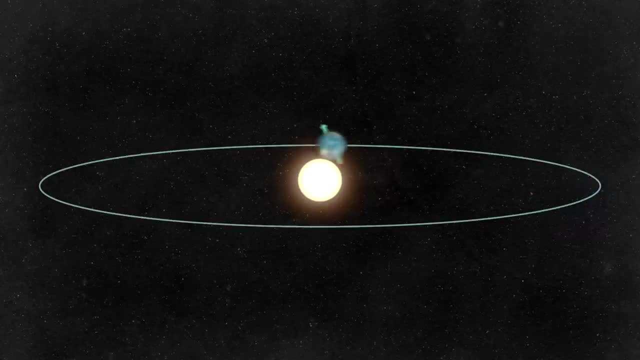 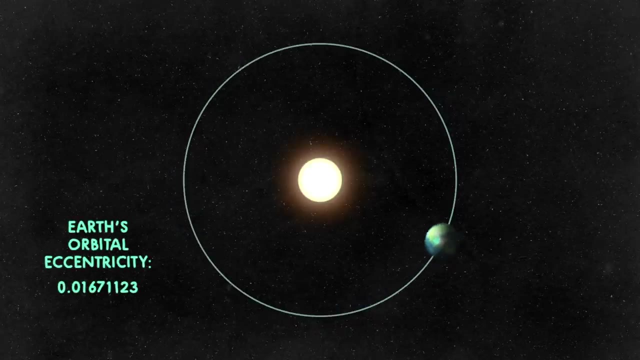 impression of how elongated our orbit is. In fact, Earth's orbit is very nearly a perfect circle. However, because Earth's orbit is technically an ellipse, it doesn't look like one and the sun isn't quite exactly at the center. it means that our distance 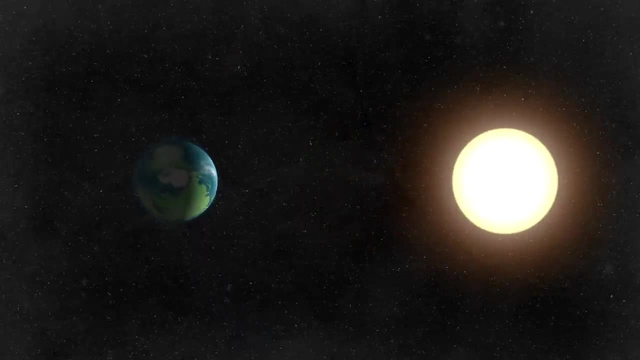 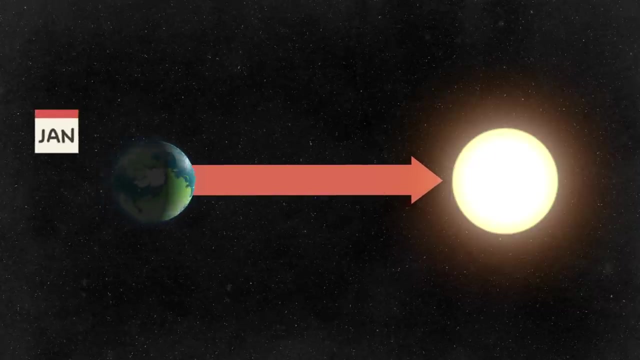 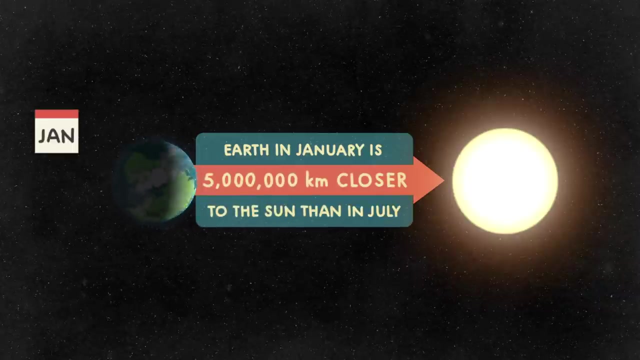 from the sun does change through the year. Aha, So winter happens when the Earth is further away from the sun. Well, no, not so fast. The Earth is actually closer to the sun in January than we are in July by five million kilometers. January is smack dab in the middle of the coldest season of 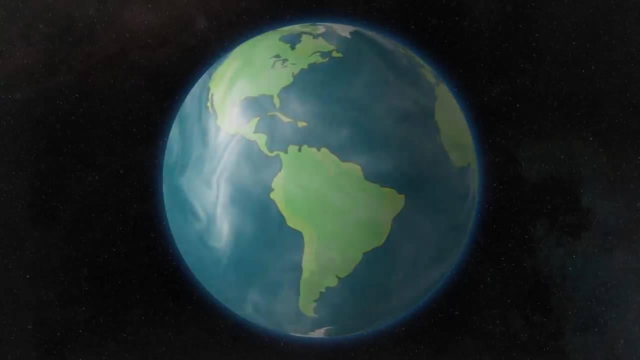 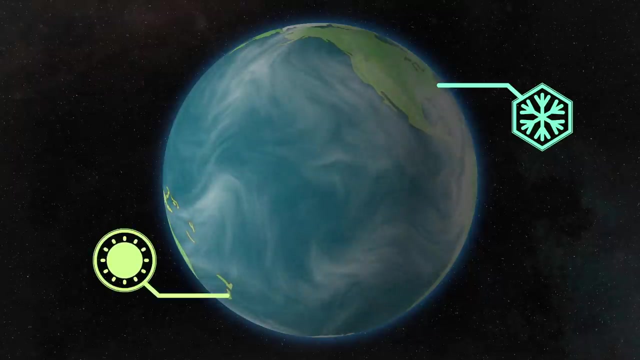 the year. for those of us up north Still not convinced, How about this? Summer and winter occur simultaneously on the surface of the Earth? The Earth is the largest part of our planet. When it's winter in Connecticut, it's summer in New Zealand. 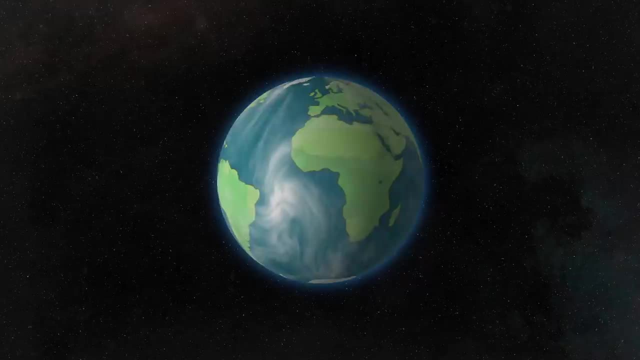 So if it's not the distance from the sun, what else could it be? Well, we need to also know that the Earth doesn't sit straight up. It actually tilts, And that axial tilt of the Earth is one of the main reasons. 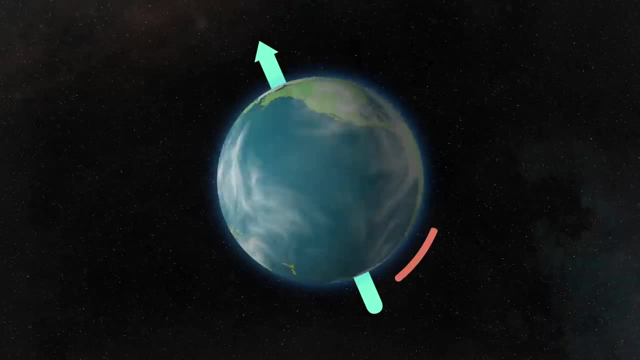 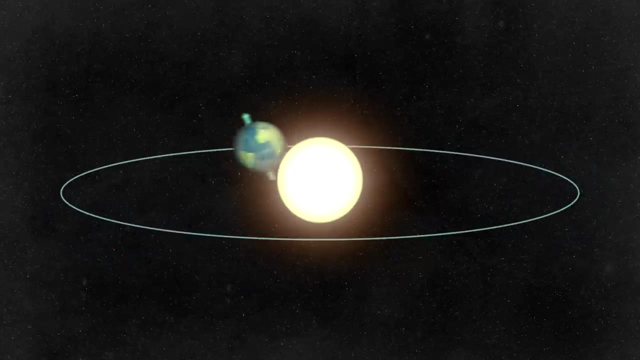 for the seasons. The Earth spins on an axis that's tilted 23.5 degrees from vertical. At the same time, the Earth revolves around the sun, with the axis always pointing in the same direction. in space. Together with the tilt, the spinning and revolving causes the number of suns to change. 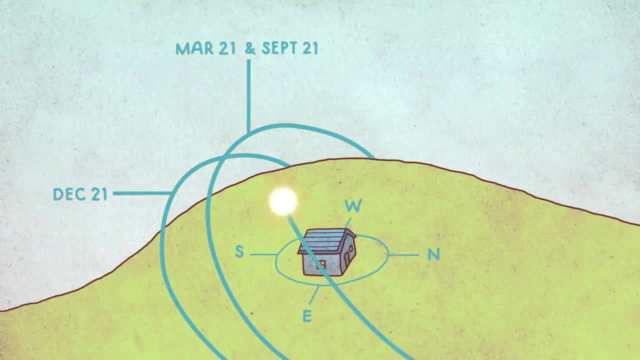 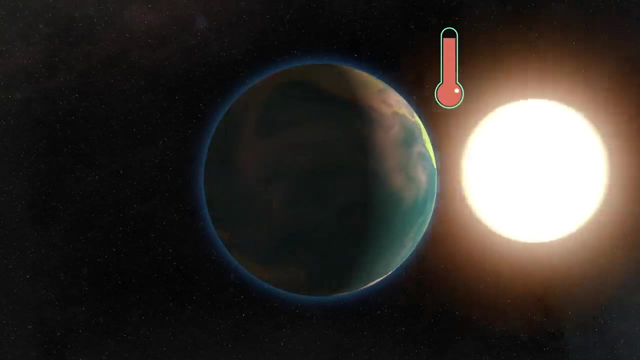 And that's because the Earth has more hours of daylight in a region to change as the year goes by, With more hours in summer and fewer in winter. So when the sun is shining on the Earth it warms up. After the sun sets it has time to cool down. So in the summer, any location that's about 40 degrees north of the 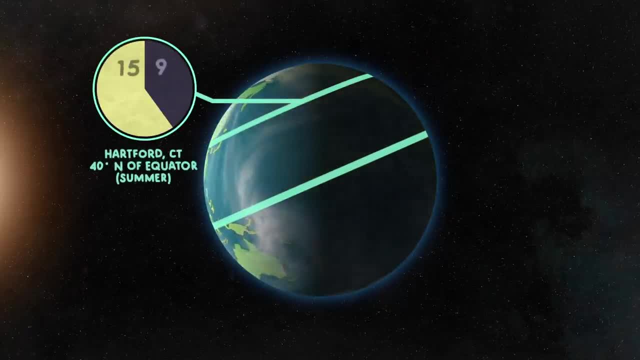 equator. like Hartford, Connecticut, will get 15 hours of daylight each day and 9 hours of darkness. It warms up for longer than it cools. This happens day after day, So there's an overall warming effect. Remember this fact for later. 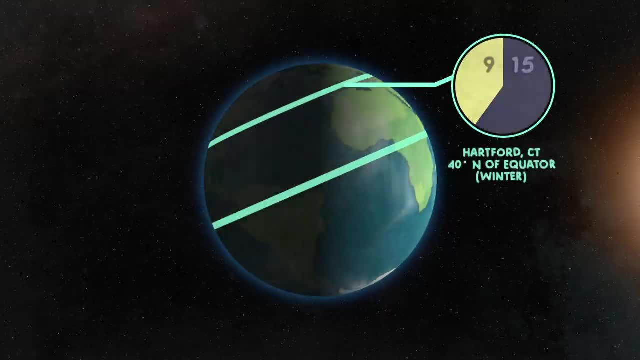 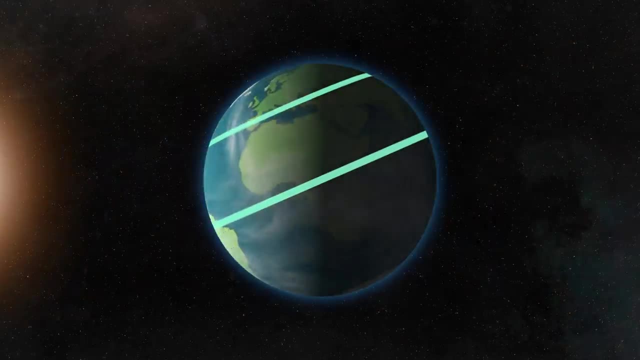 In the winter, the opposite happens. There are many more hours of cooling time than warming time, And day after day this results in a cooling effect. The interesting thing is, as you move north, the number of daylight hours in summer increases. 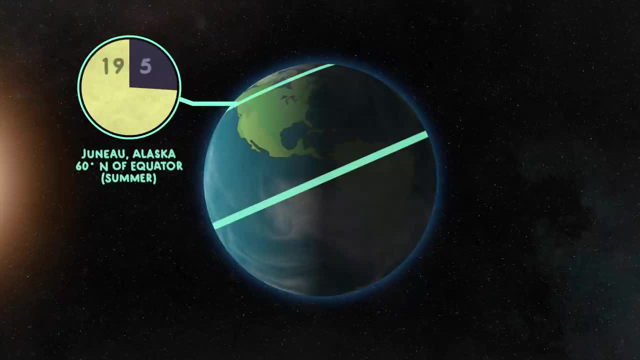 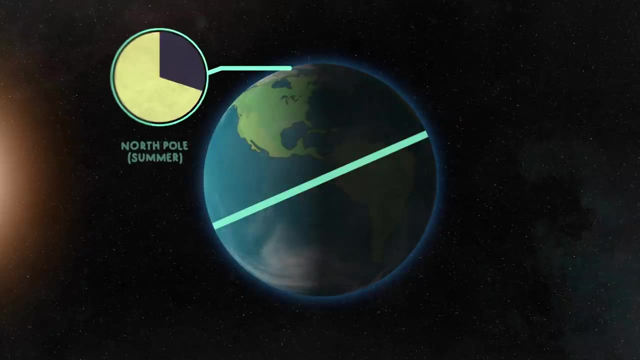 So Juneau, Alaska, would get about 19 hours of daylight on the same summer day that Tallahassee, Florida, gets about 14.. In fact, in the summertime at the North Pole, the sun never sets. Okay, then, it's all about daylight hours. I've got it. 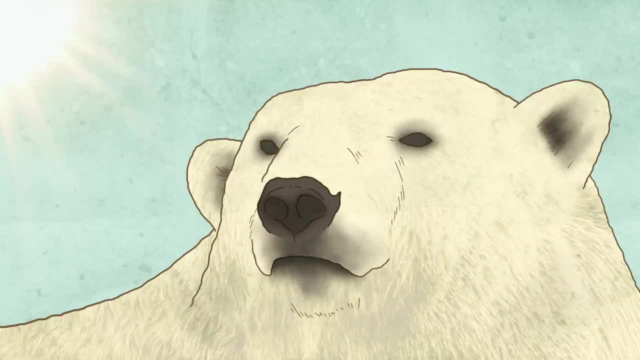 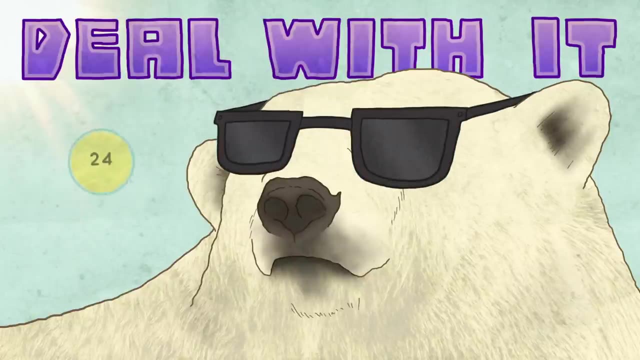 Well, no, There's another important piece to this puzzle. If daylight hours were the only thing that determined average temperature, wouldn't the North Pole be the hottest place on Earth in northern summer, Because it receives 24 hours of daylight in the months surrounding the summer solstice? 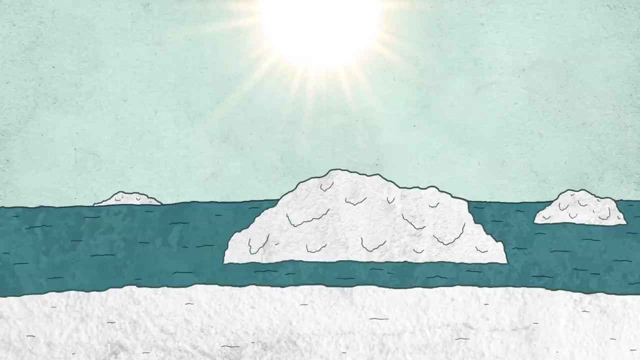 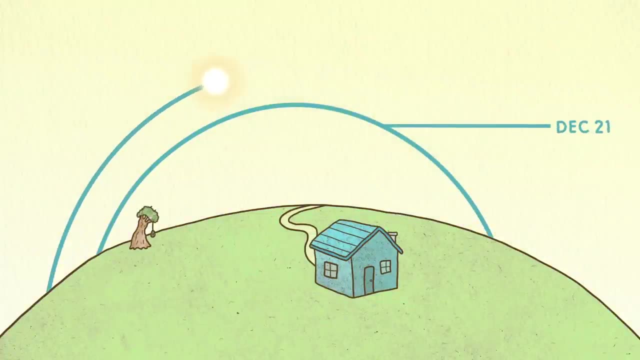 But it's the North Pole. There's still icebergs in the water and snow on the ground. So what's going on? The Earth is a sphere, and so the amount of solar energy. an area receives changes based on how high the sun is in the sky. 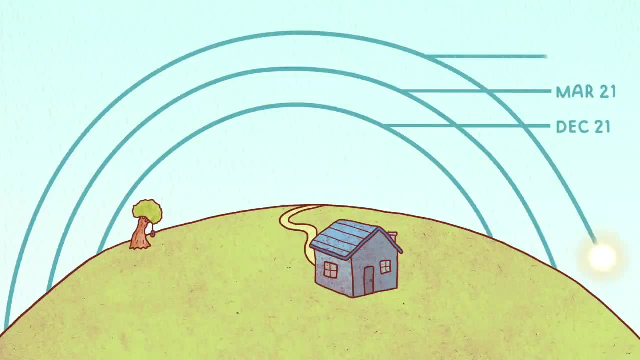 which, as you know, changes during the day between sunrise and sunset, But the maximum height also changes during the year, with the greatest solar height during the summer months and highest of all at noon on the summer solstice, which is June 21st in the Northern Hemisphere and December 21st in the Southern Hemisphere. 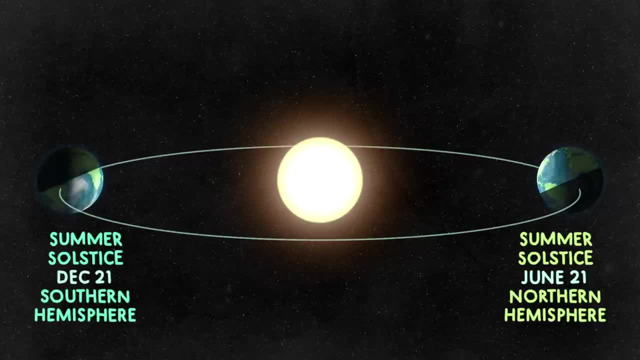 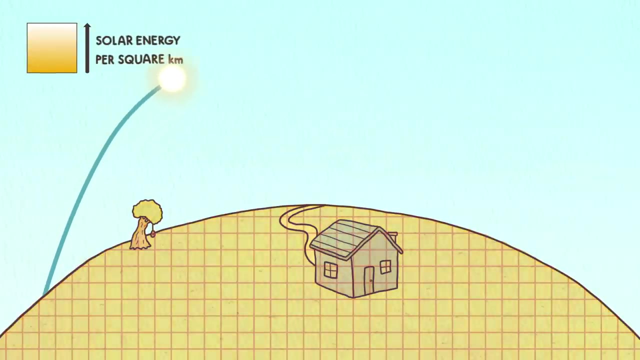 This is because, as the Earth revolves, the Northern Hemisphere ends up tilted away from the sun in the winter and toward the sun in summer, which puts the sun more directly overhead for longer amounts of time. Remember those increased summertime daylight hours. Solar energy per square kilometer increases as the sun gets higher in the sky.